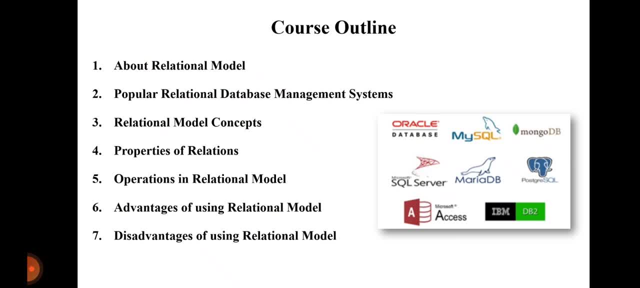 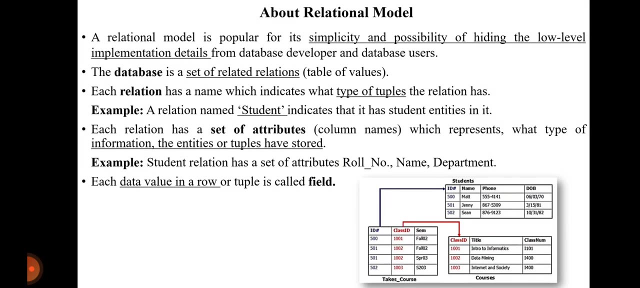 then relational model, concepts, properties of relations, then operations in relational model, advantages of using relational model and disadvantages of using relational model. These all points will be covered in this session, So let's start. So the first point is about relational model. What is meant by relational model? right? 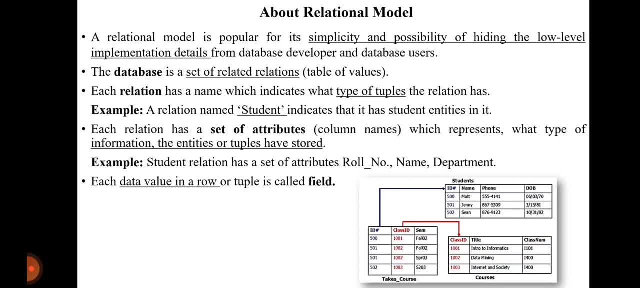 So at that point we know that what is meant by model. okay, Model means just representation, Representation of particular information. So relational model is popular for simplicity and it has also possibility to hiding low level implementation details with database. okay, 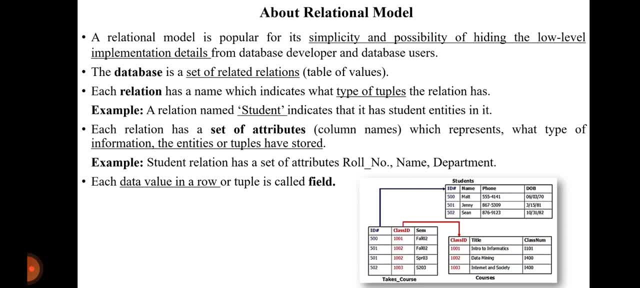 So relational model simply means collections of tables and it shows the relation between that tables. This is the concept of relational model, right? What is meant by database? We know that database means collections of tables, right? So set of relations. 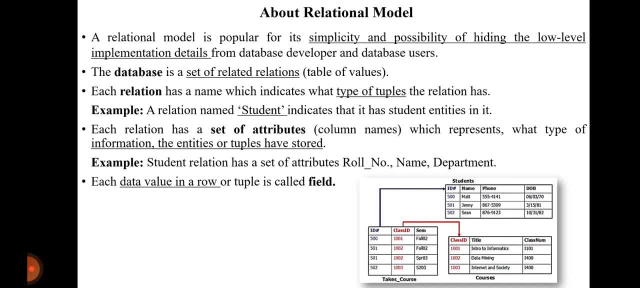 We know that it will hold so many related relations between that particular tables. this is called as relational model, So every relation has a particular name. See, in this table, this table stores the details of students right. First table shows the details of students personal details. then another table shows the course details, right. 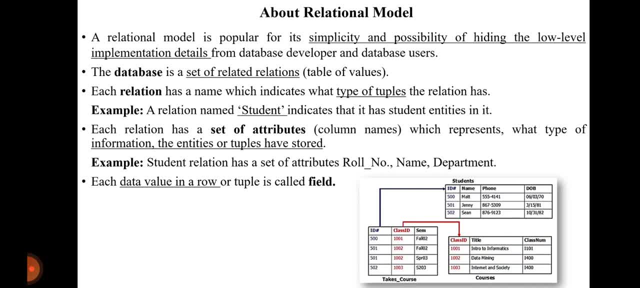 So the relation is. student Means the particular database or particular table, students. So student is one database and there are multiple relations of that particular students will be stored. So every relation has a set of attributes, right, Student? student is one. 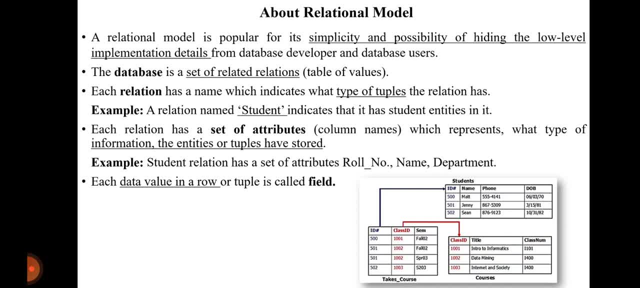 relation and student has different specifications or we can say attributes. So the attributes mean their ID, name, phone number, date of birth, etc. So this is called as particular relational model, means there is relationship between each and every tables and this all set of tables are stored. 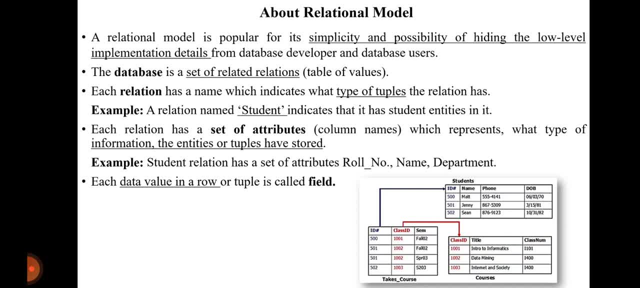 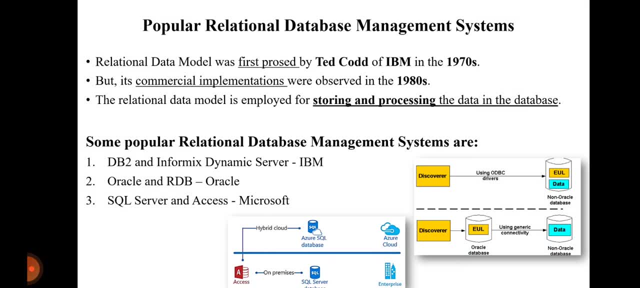 into the database right? This is the concept of relational model. Next, the next point, is there are some popular relational database management system. So before that, first, when relational database management system have developed. So relational data model was first proposed by 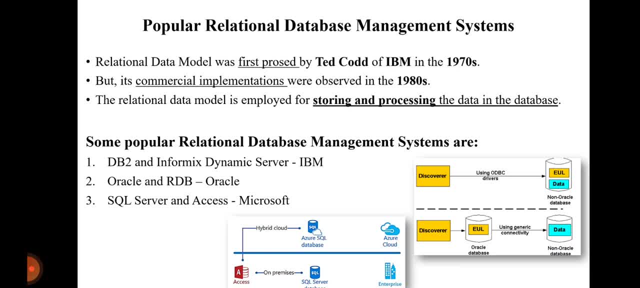 Ted Kord of IBM in 1970. And their commercial implementation were observed in 1980.. So relational data model is generally used for to storing and processing different data in database And also there are some popular relational database management system like for IBM DB2 and Informix dynamic server. This is own. 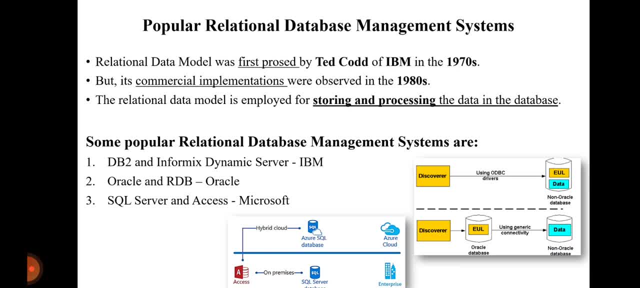 IBM relational database management system The complete details and complete information of the particular related to the IBM. This information will be stored into this database, Then Oracle and RDB. These are the some relational database by the Oracle, Then SQL server and access this database provided by the Microsoft. So this is. 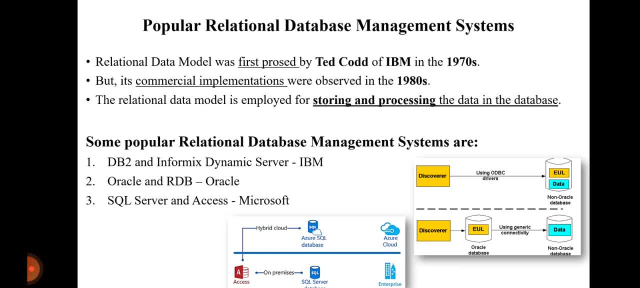 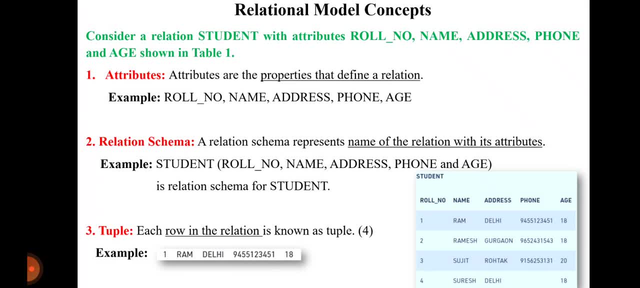 called as relational database, And that will be a real life database generally used. okay, Next, the next thing is relational model concept. So this relational database have a particular or some concepts regarding the particular tables? okay, So, for this concept, just consider this table. okay, The table name. 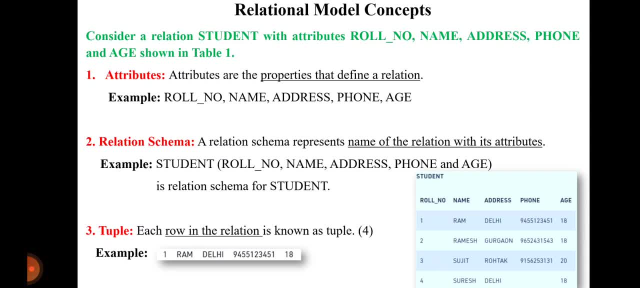 is student. So the first concept of relational model is attribute. What is meant by attribute? Attribute means specification, okay, Attribute of students. So student attribute are roll number, name, address, phone and age right. So attributes are the property that define a particular 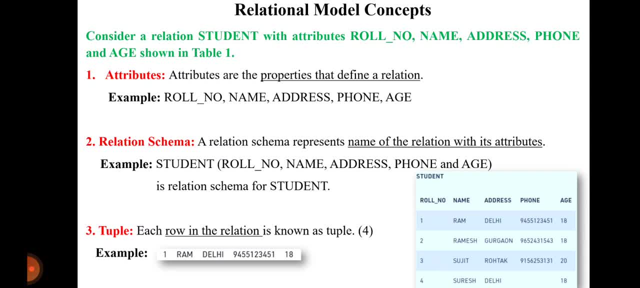 relation. So these are called as attributes. The next concept is relation schema. So relation schema means the name of relation and name of the attributes and combinations of that. For example, name of the relation is student and name of the relational attributes are role number, name, address, phone and age. 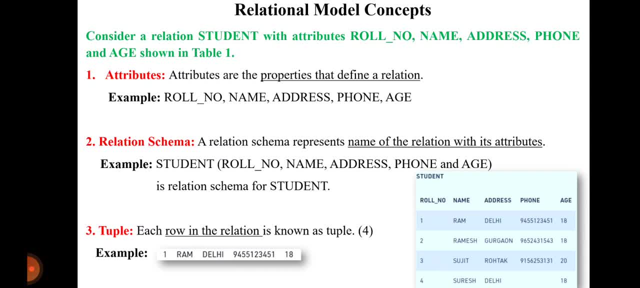 So the combination of these relations and the relations attributes, this is called as relation schema. Next concept is tuple. So tuple simply means each and every row in particular table. Okay, So this is called as tuple. So in this table there are total four tuples Right. Each row in the relation is called as tuples. 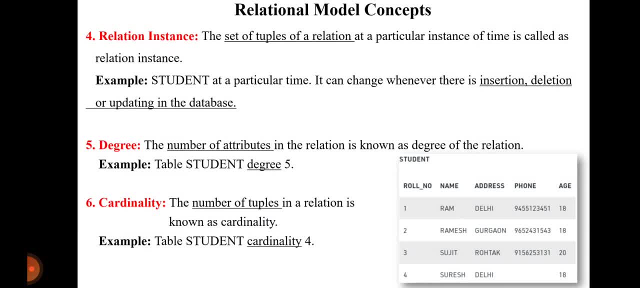 Next, The next concept is relation instance. So relation instance means set of tuples of particular relations, in particular instance at a time. Okay, See, in this table That is student table. Okay, So in this student table there are total four rows and total five columns, Right? So this information will be dynamic, not a fixed information. 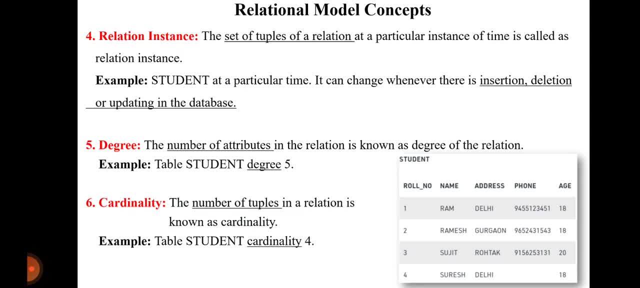 Right, You can insert different data of the student, You can delete those data, you can modify or update those database, Right? So this is called as relation instance Means every relation instance is a dynamic, not a fixed one. Okay, Next concept is relation table: Degree. So what is mean by degree? 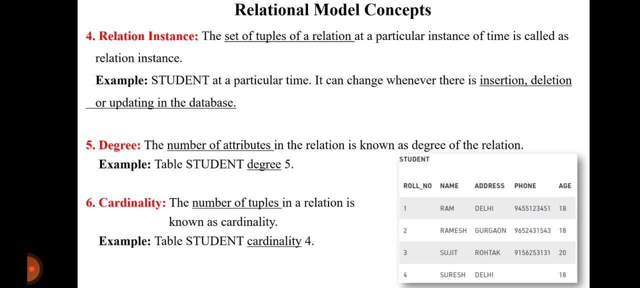 Degree means total number of attributes of that particular relation. This is a degree of that relation. So here relation is student And student has total five attributes: Role number, name, address, phone and age Means degree of student is five. Next one is cardinality. Cardinality means number of tuples in that particular relation. 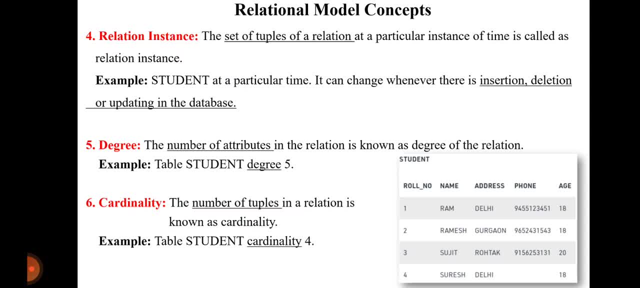 So in this table, student- So student- has total five attributes. So cardinality means four rows. Okay Means that four tuples, Or we can say cardinality of the student is four. So cardinality means number of tuples. You must remember this thing For your online examination. also, Degree means number of attributes. 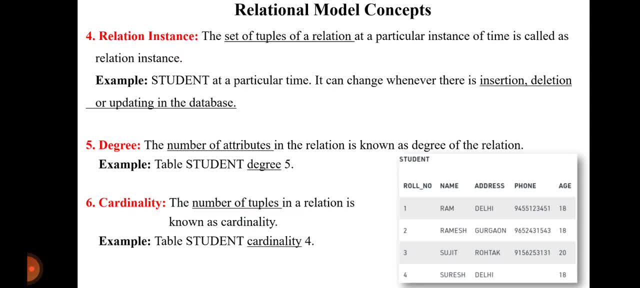 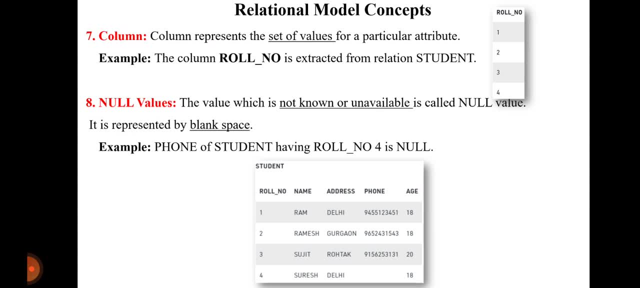 And cardinality means number of tuples. Next, The next concept is column. We all are familiar with this concept. rows and columns, Right Column, represent a particular set of values For particular attribute, For example, role number. Role number is a specific column And it shows, and it stored, similar types of information. 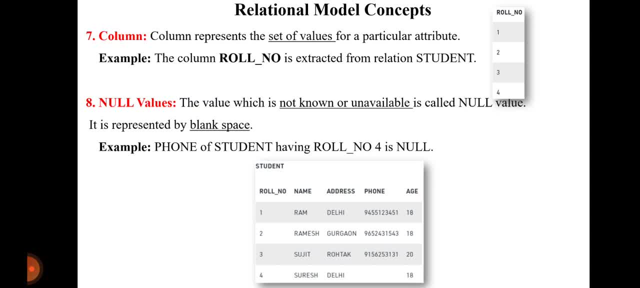 Right. Next and last concept is null value. So what is mean by null value? There is a value which is not known Or unavailable. This is called as null value. Okay, And null value is represented by the blank space. See here in student table, In the phone column. Okay, 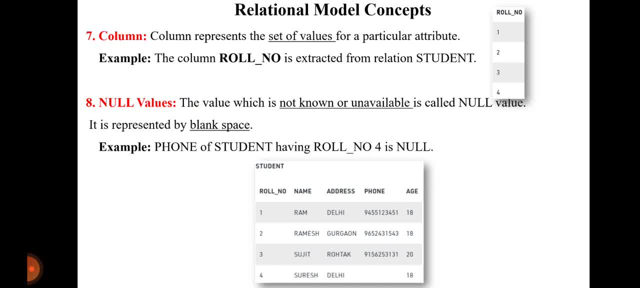 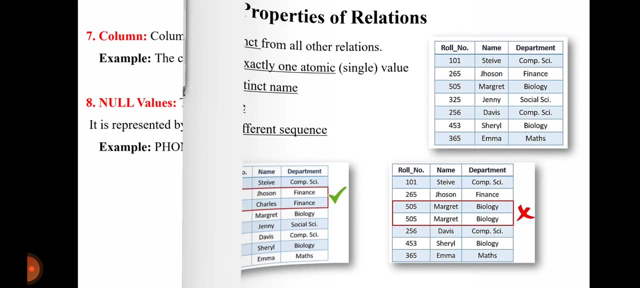 In the phone of student Having role number four is null. Right Role number four Phone number is null. Null means the particular information is unavailable, Clear. So these are the some concepts of relational model. Next, Now, there are some properties of relational model. While designing a particular relational model, 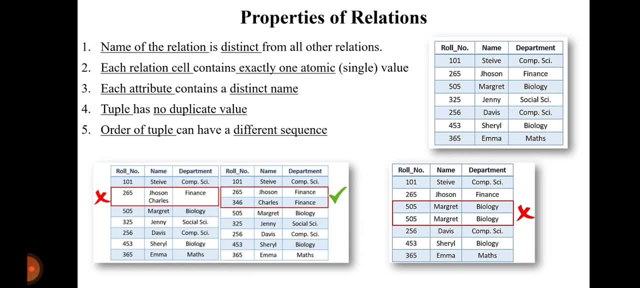 You must follow some properties, Okay. So the first property is Name of the relation is distinct from all the other relation. So in this example, student Student is one unique name, Okay, And this is a particular name of that particular relation. Okay Means the particular table or particular database stored complete information of student. 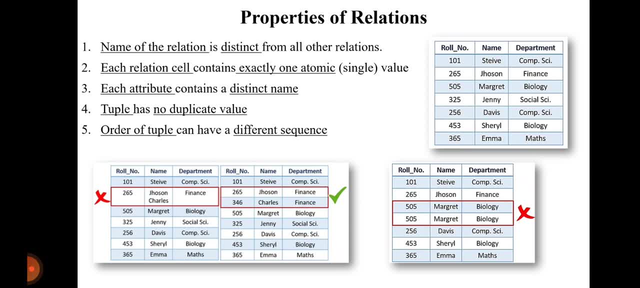 So student is a unique name. Next property is: Each relation cell Contains exactly Only one atomic value. See in this first table, Role number 265. Okay, This stored. There are total two students name, That is Johnson and Charles. So this is not allowed In relational table. Every field in particular table. 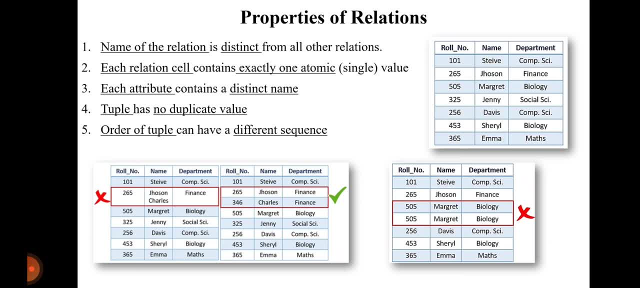 Stored only single value Or atomic value. Right. Next property is: Each attribute contains a distinct name. Each and every values has The particular unique name. Okay, Not a duplicate value. So see in this second table, Role number 505. Okay, And the name is Magrat. Okay, So these are the some duplicate values. 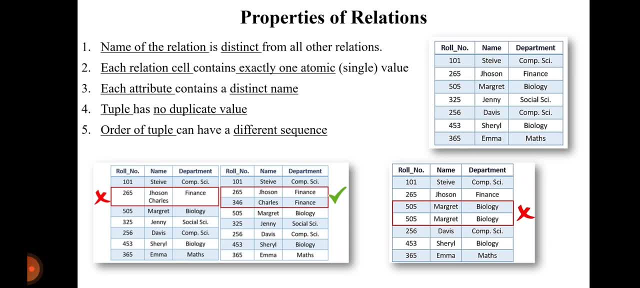 Or duplicate rows will be available. So tuple has no duplicate values. Right And order of tuple can have a different sequence Means every information will be stored And the particular sequence wise, Either in ascending order Or in descending order, Means all the information in particular sequence In supervised manner. 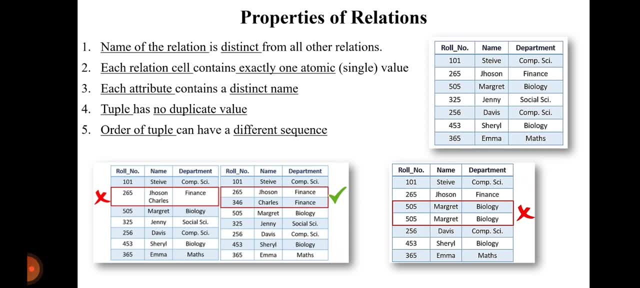 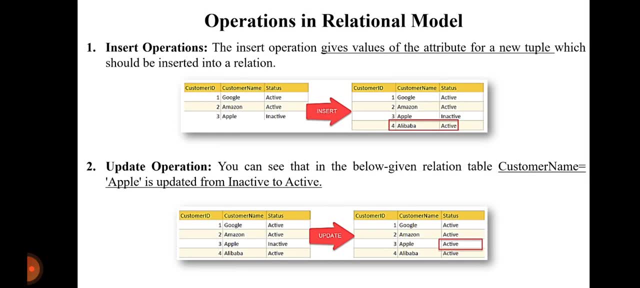 Right Next. So the next point is Operations in relational model. So we know that There are some basic operations Like insert, Update, Delete And select. So these operations We will perform On the relational model And for that purpose We will use Different queries. Right So how We will apply. 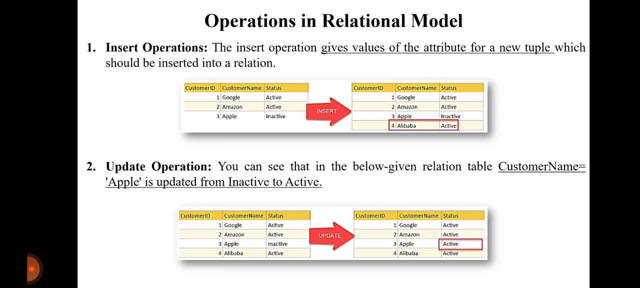 Different queries On database I will explain In my next session Or in my next videos. Okay, So, So. So The Here is only A theoretical part. So first one is Insert operation. Insert operation means To add or insert New value Or new information In the particular table, See here. 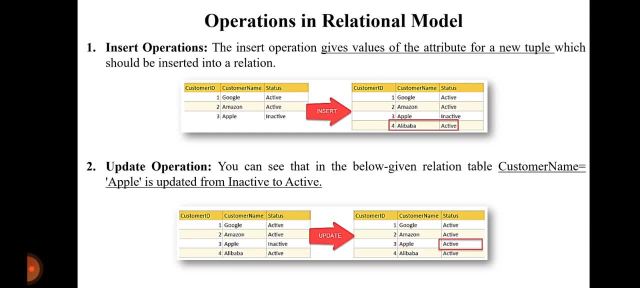 The first. There are total Three rows Are stored And here New information regarding Alibaba Customer name: Okay, This information will be added into the Particular table. Next one is Update. Update means Modify the particular information. Okay, okay, see here. the customer name equal to apple is updated from inactive to active state: see here. 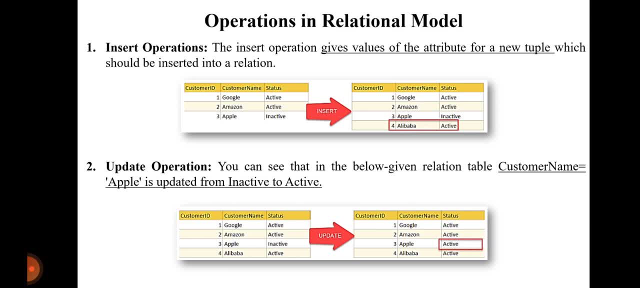 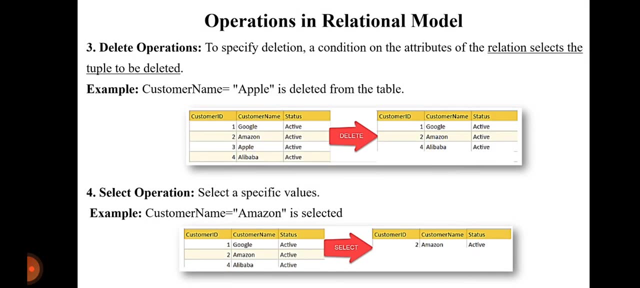 in first table the apple customer name and their status is inactive. but after updating is performed, the customer name is apple, their status is active. so update means modify those data. okay. next and the next operation is delete operation. delete operation means simply remove the particular tuple in that particular table. okay, you simply delete the particular customer name, that is apple. 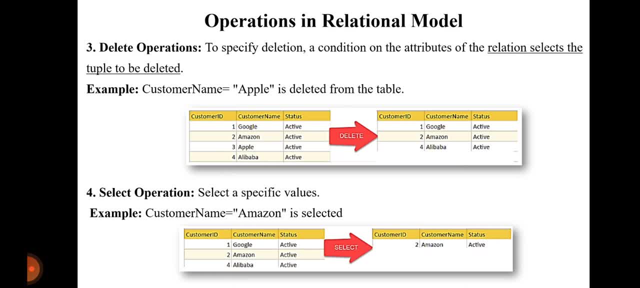 okay, so delete those particular row. next one is select operation. so select operation generally used for to select a specific values in particular table. for example, customer name is amazon, right, so particular amazon, this row only selected. so these are the different operations. that operations will be performed by using different queries or sql queries. okay. 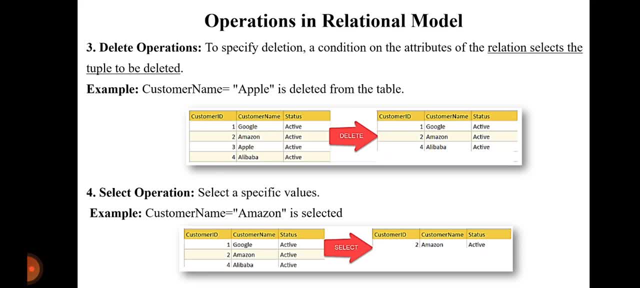 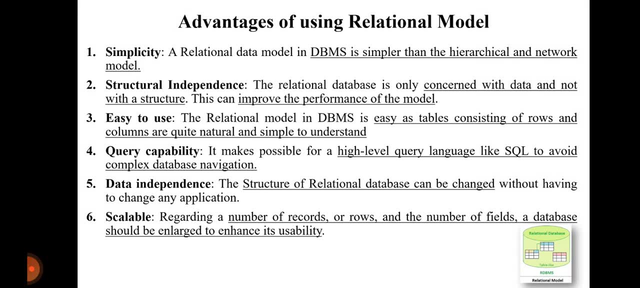 we will see this information or this concept in my next video. now the next point is advantages of using relational model. so these are the some advantages. first one is simplicity. relational model is most simpler than hierarchical and network model. so what is mean by network and hierarchical model i have already explained in my last video. okay, 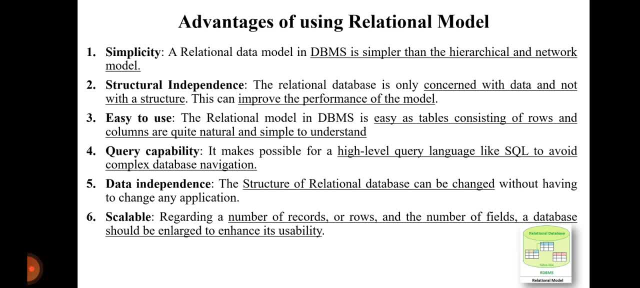 so relational model is most simpler as compared to that model, because relational model you can use it in a table format or in tabular format like rows and columns, right, so it's very simple. next one is structural independence. the relational model is concerned with data only, not with this. 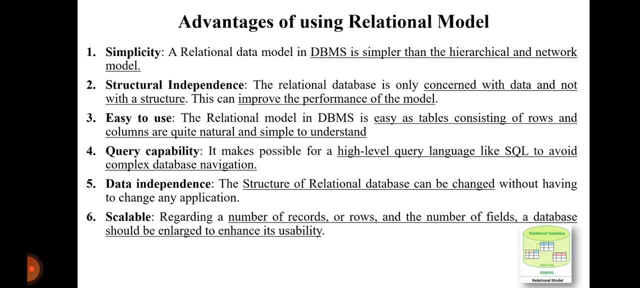 structure: right, because relational model or tables, we will store only atomic value. we will not store any duplicate value, right, so it concerned with data only, not with the structure. so this can improve the performance of model. The next advantage is easy to use because database management system. there are collections of tables like rows and columns, So it's quite natural and simple to understand. Next advantage is query capability. Relational model always use high level query languages like SQL, right, So they avoid a complex database navigation. 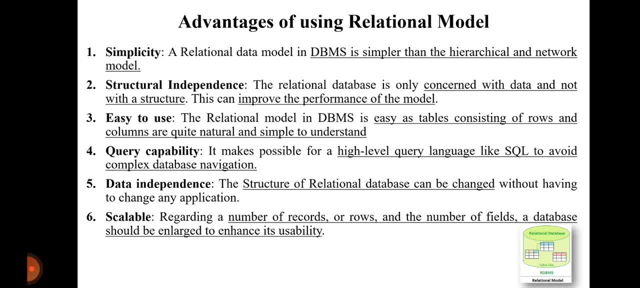 Next, data independence. So structural of relational database can be changed without having to change any application. We will insert, update, delete and modify those database right, So that will be a data independent or flexible way. Next one is scalable. Scalable means simply the number of records, number of rows, number of fields and also database should be enlarged or enhance its usability. 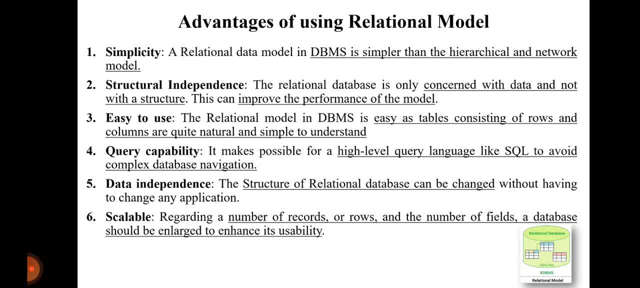 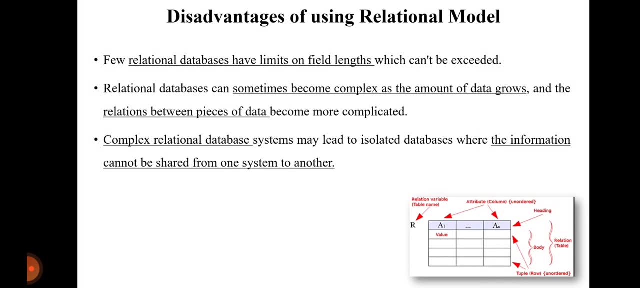 As per the customer requirements, we will add the different data, We will add different information, We will remove the information from the table, So that will be a completely scalable or flexible. Next and the last one is disadvantages of using relational model. So there are some few relational database have limits on field length means, for example, there are only a 10 digit number will be stored. 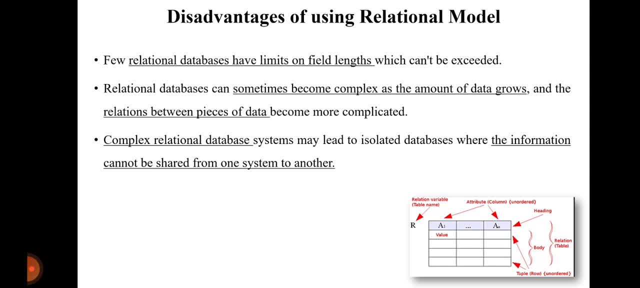 So this is a limit, okay, because there are some relational database model have a particular field length, limited field length. So this is the disadvantages of that Next. Next, some relational database can sometimes become a complex because there are large amount of data will be stored, right. 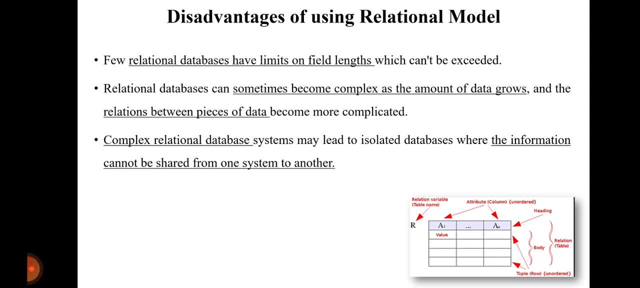 Next one is complex relational database system. So this database system information cannot be shared from one system to another. So this is also disadvantages, because we will share this particular tabular information with others. employees also right. So these are the some disadvantages using relational model. 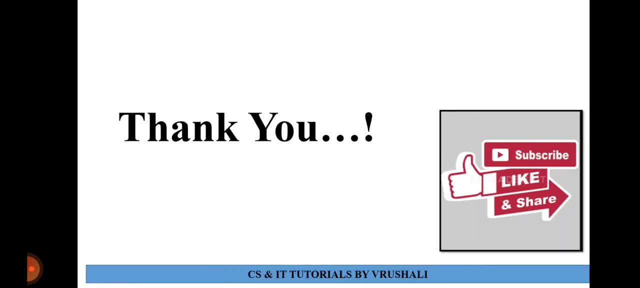 So this is a complete introduction about relational model. in my next video we will learn about some integrity constraints and some ER models with query. So after watching this video, please subscribe my channel and also share with your friends. Keep practicing, Thank you.